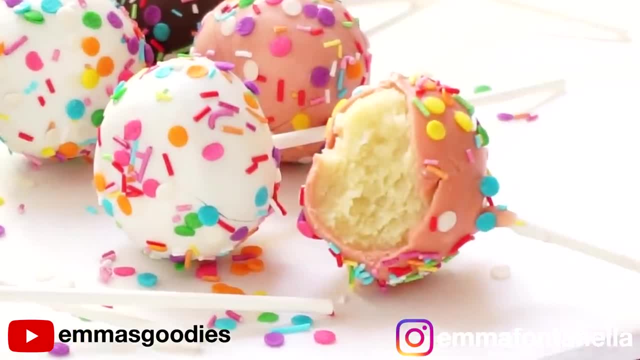 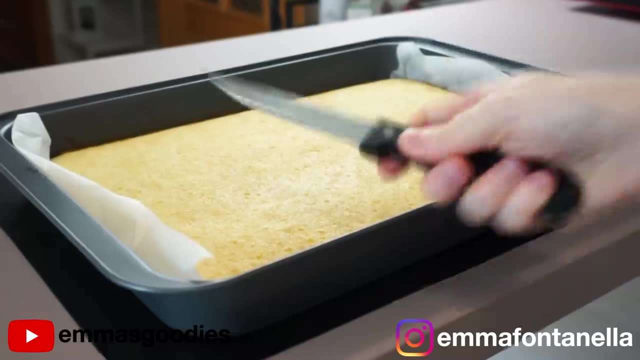 Cake pops are amazing. They're usually made with cake scraps. but what do you do if you don't have leftover cake? You'll have to bake one off yourself and wait for it to cool. Most importantly, why would you spend an hour of your time making a beautiful cake to only destroy it? I'm going to 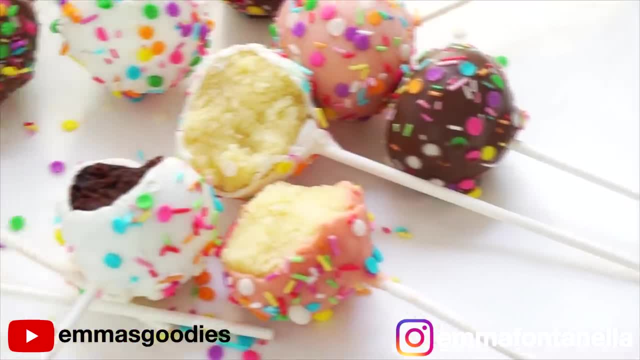 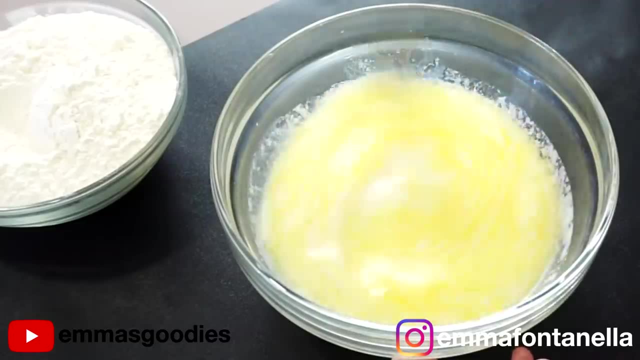 show you today the easiest and fastest way to make fresh, delicious cake pops when you don't have leftover cake. We're making my mug cake recipe today. quadrupled To the melted butter and vanilla, I've added sugar and milk. Give these a quick mix and add the flour baking powder. 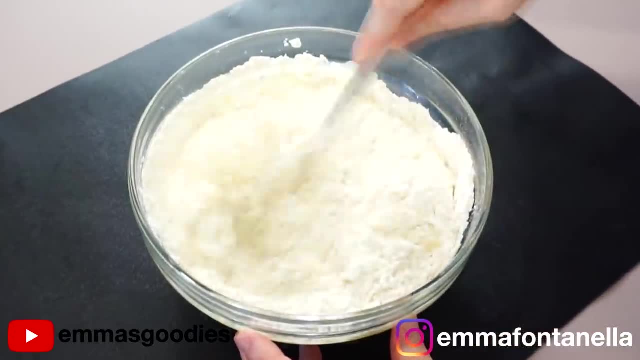 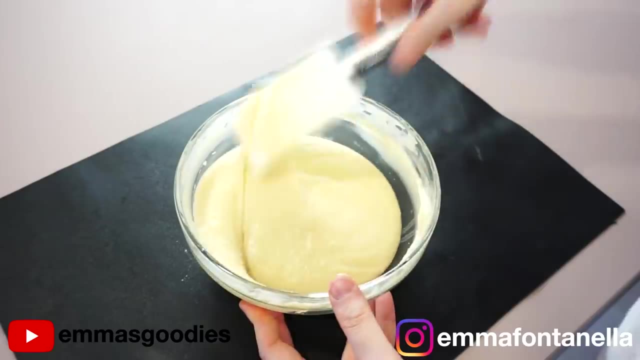 and salt. If you've ever made my mug cakes, you're familiar with this recipe and you know how easy and delicious these are. Do not use a fork to mix the batter. I had to switch to whisk, as it's much faster and easier to combine everything and it really breaks up those. 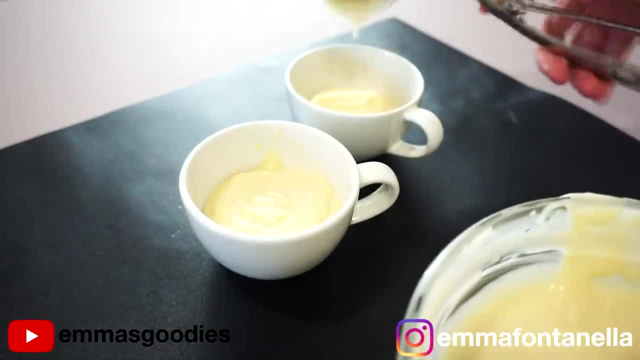 flour lumps. You're going to pour half of the cake batter in two mugs, or I should say, in my case, teacups. With the other half of the batter, we're going to make a chocolate cake, a chocolate mug. 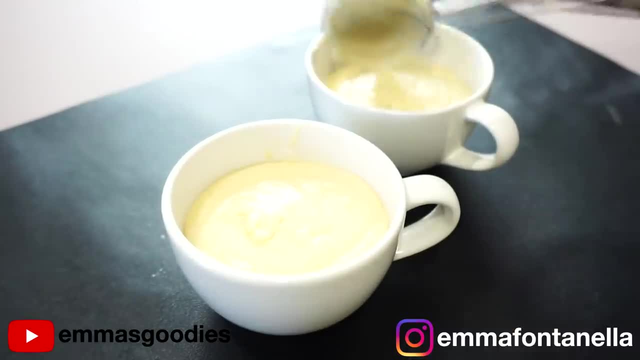 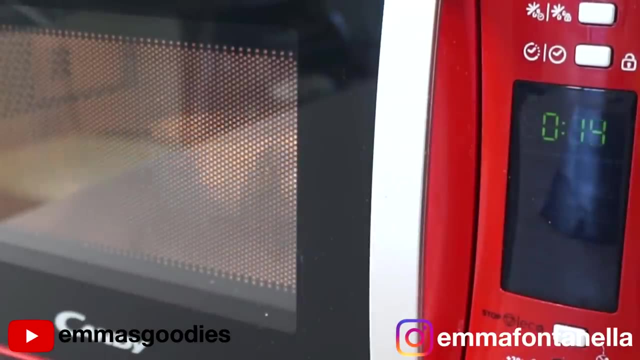 cakes in just a second. Now you don't have to use mugs, You can just use one microwavable container. However, because I wanted the name of this video to be one minute cake pops- one minute cake pops it's gonna be, because my cakes take one minute to cook If you are using just one container. 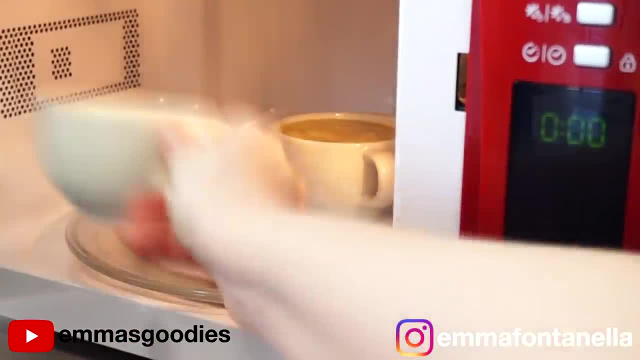 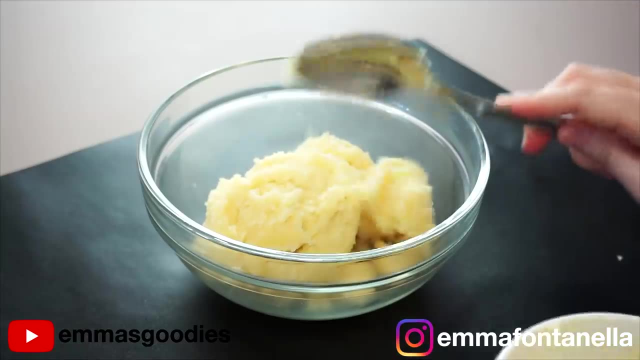 please know the timing will vary If you're using mugs or cups. cook these on high for about a minute to one minute and 30 seconds. Now, at this point, you're going to have one of the biggest, most important dilemmas of your life. It's going to be a true existential crisis, and that is 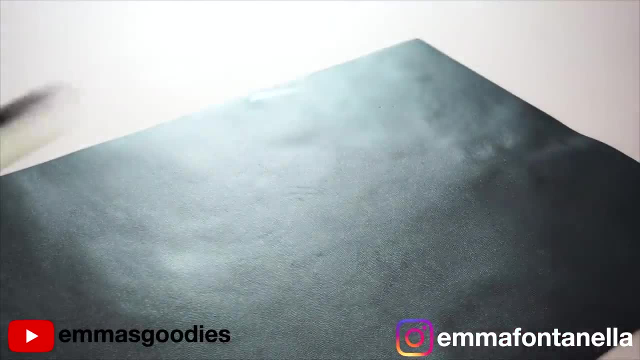 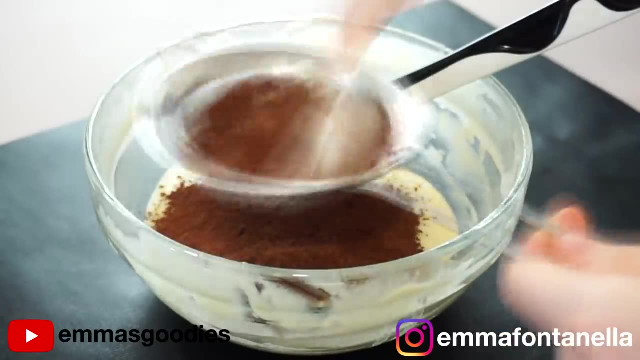 do I just need the mug cakes or do I make cake pops? I'm going to go with cake pops because so many of you asked That aside, and let's make the chocolate mug cakes. To the batter add some cocoa powder, which you do want to sift to avoid over mixing, and some extra milk By the. 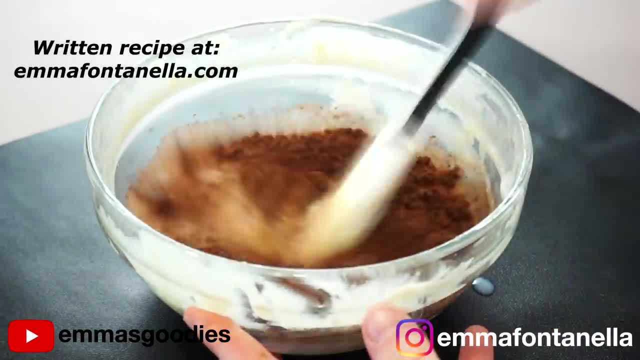 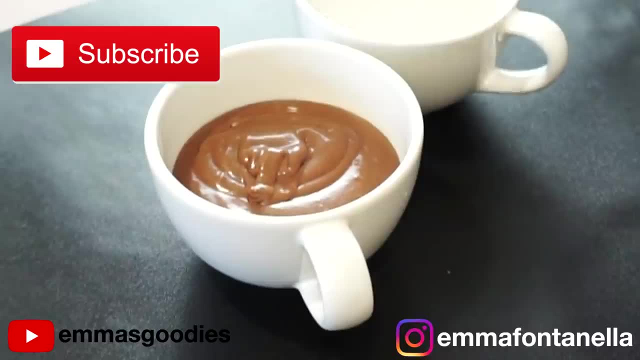 way. the full written recipe will be in the description box and on my website, And if you're new to my channel, hello there, welcome. Make sure to subscribe and click that bell. I post new videos every week. Transfer the batter into mugs and microwave again for anywhere between a. 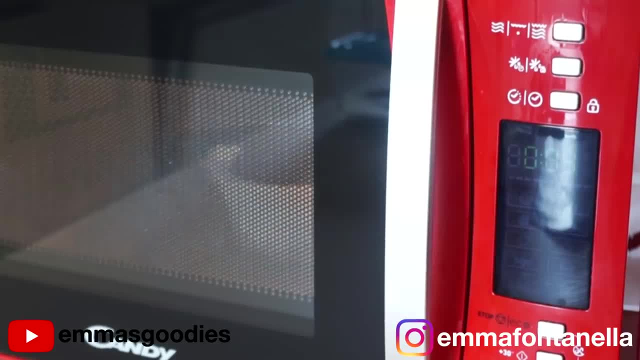 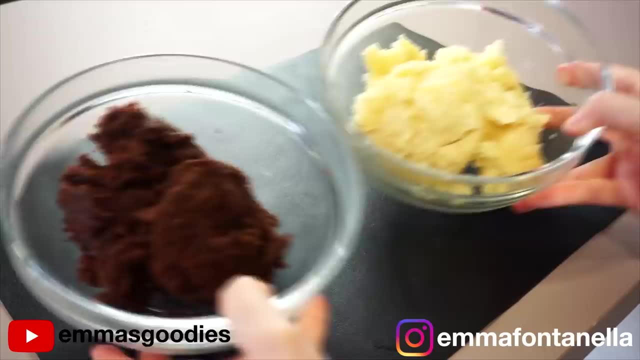 minute to one minute and 30 seconds. Now, what I love about making cake pops this way is that the cakes cool fairly quickly So you can move on to making the cake pops straight away. You don't have to wait half an hour for these to cool like a regular cake. Obviously careful: Do not burn. 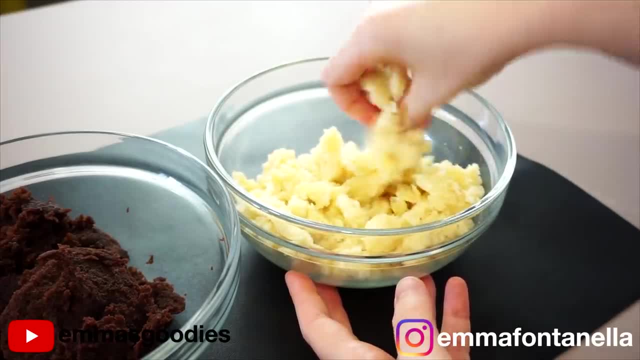 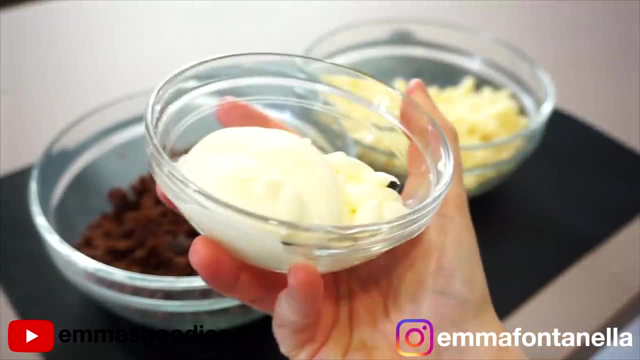 yourself. Let these cool slightly, I'd say for about five to 10 minutes at the most, and break up that cake using your fingers. Now let's talk frosting. I'm using some leftover buttercream that I made for my lunchbox cakes. Do I expect you to make a teeny little bit of frosting for? 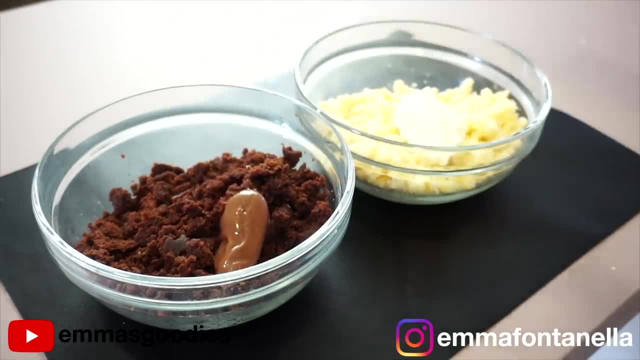 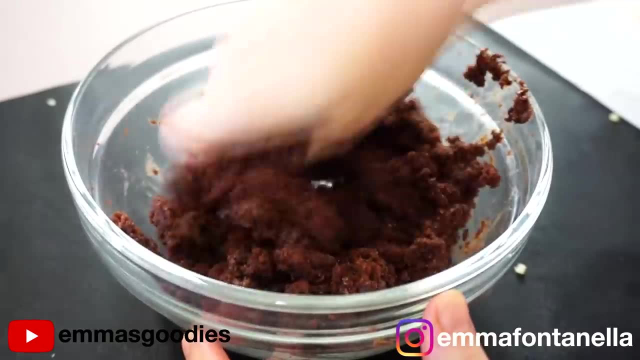 one minute cake pops? No, of course not. What you can use for the vanilla cake pops is marshmallow fluff. I've tried it and let me tell you it is better than using buttercream. It's amazing. You could also go with cookie butter- absolutely delicious- or Nutella, which is what 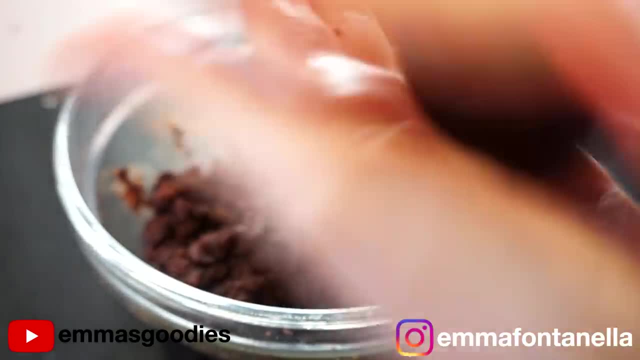 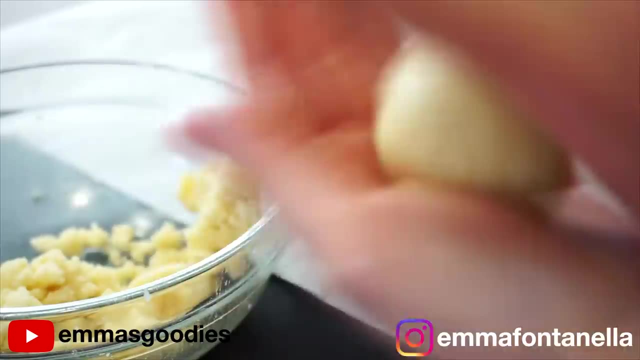 I'm using for the chocolate cake pops. If you've never had chocolate Nutella cake pops, honey, this is your chance. So good And my absolute favorite: chocolate cake, Nutella and white chocolate coating. It's the best combo ever. I'm telling you Now the amount of frosting you'll 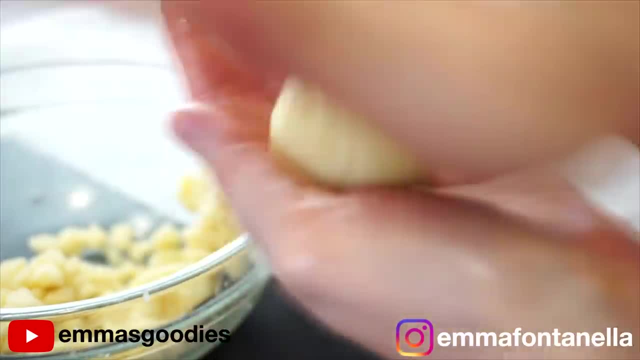 need really depends on what type of spread and frosting you use. If you're using chocolate, you're going to need a little bit of chocolate. If you're using chocolate, you're going to need a little bit of chocolate. You'll need about two to three tablespoons. You just want those cake. 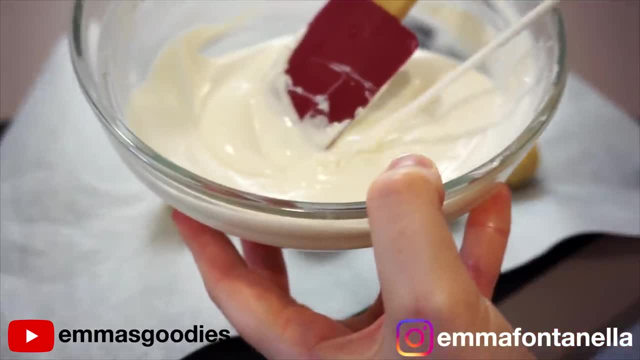 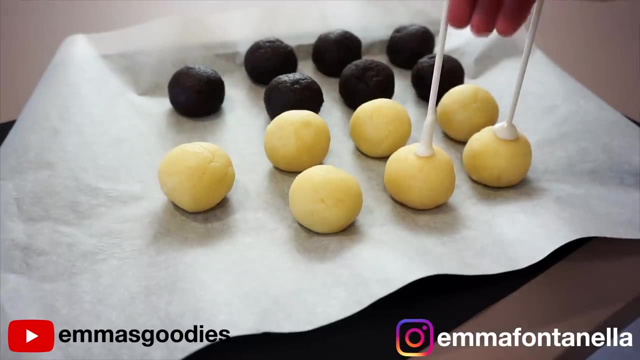 crumbs to stick together and form cake balls. Place your balls onto a tray and we're going to turn them into cake pops. with some sticks, You're going to stick each stick. you're going to stick each stick into some melted chocolate of your choice and then into your mini cakes. Now, these 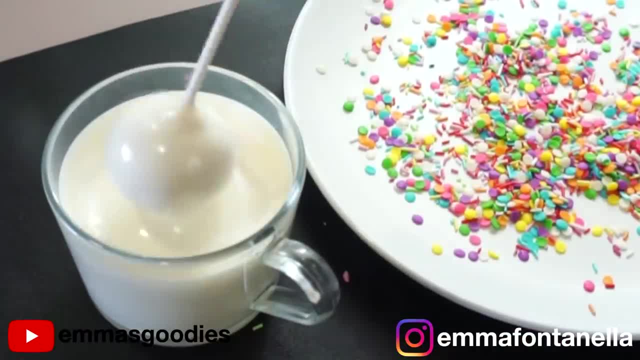 have to go in the freezer for about 10 minutes. We need that chocolate around the stick to fully harden. That way the cake pop stays put when we dip it into the melted chocolate. I'm using plain melted chocolate to get a little bit of that chocolate flavor. I'm going to add a little bit. 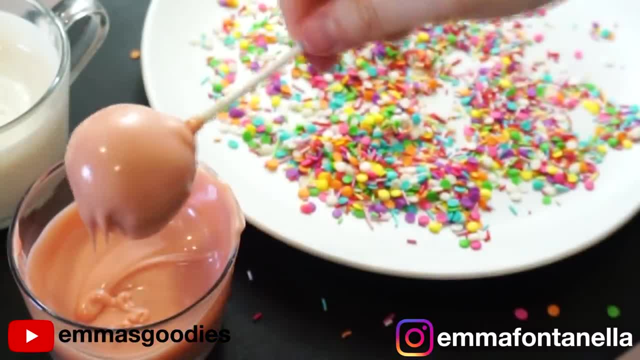 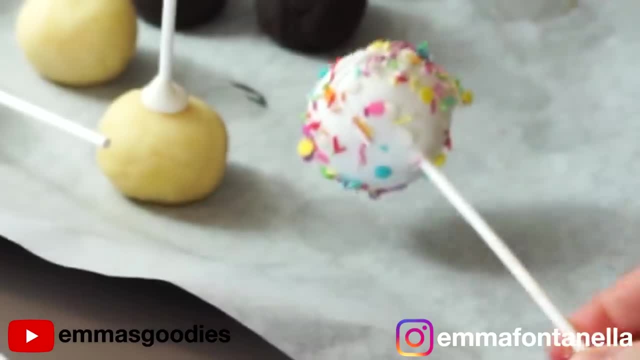 of coconut oil. I'm going to add a little bit of coconut oil. I'm going to add a little bit of coconut oil. Now, if you have one of those fancy cake pop stands, use it. If you're cheap, like me, and you don't want to get one, just place these onto some parchment paper. It does the job. 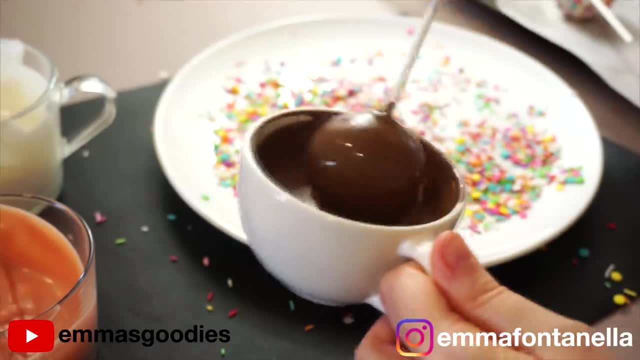 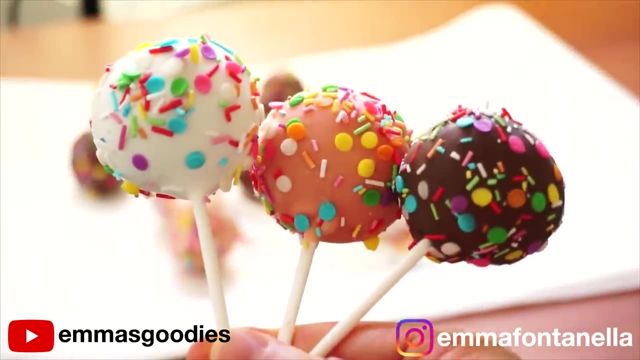 perfectly. These should set up pretty quickly, especially with the coconut oil. If they're not setting up as fast as you'd like, just pop these in the fridge for about five to 10 minutes. Now, this doesn't need to be said, but these are pretty amazing. There's something so nostalgic.